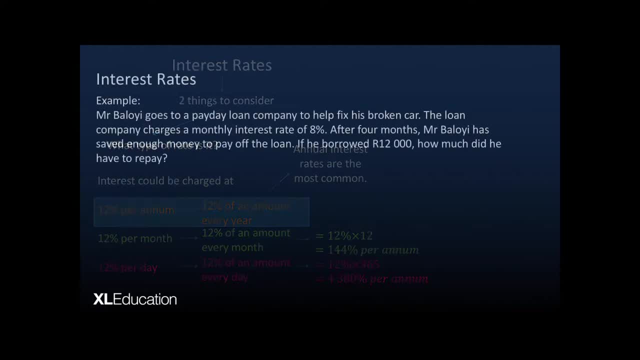 interest rate. that is usually something quite out of the ordinary. So let's look at an example. Mr Baloyi goes to a payday loan company to help fix his broken car. The loan company charges a monthly interest rate of 8%. After 4 months Mr Baloyi has saved enough money. 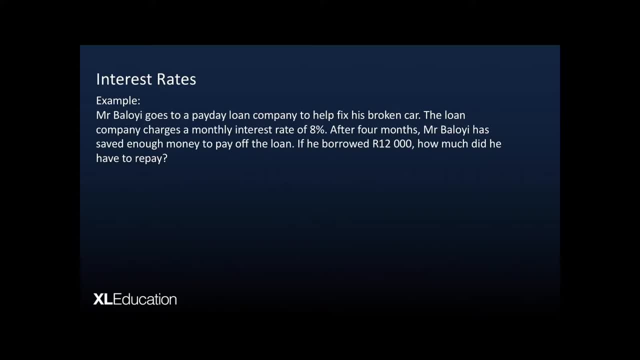 to pay off the loan. If he borrowed 12,000 rand, how much of that interest rate would he have to repay? So we're going to use our formula for compound interest. but we note now that the interest rate is a monthly interest rate. So we've got 8%, but our period of 4 months means we 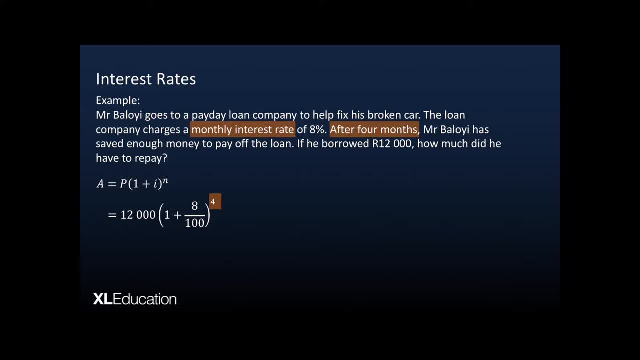 have to use an exponent of 4, because interest is calculated 4 times, because it's a monthly interest rate over 4 months. And we find then that after 4 months he has to repay 16,000 rand, so that is 3,325.87.. So usually if you get a monthly interest rate or even a daily 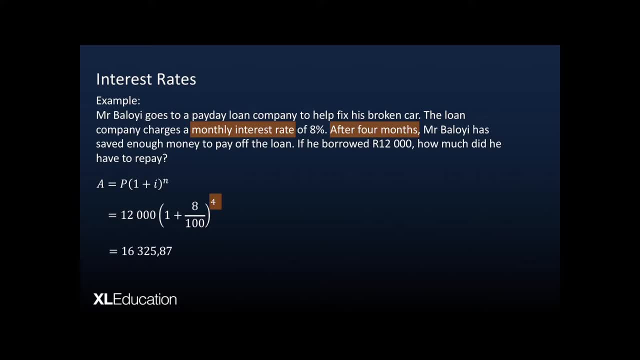 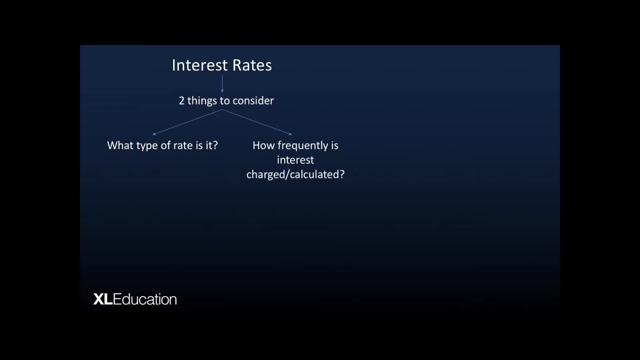 interest rate. chances are you are dealing with a Loan shock or some other disreputable interest rate. So then the other thing we have to consider is how frequently interest is calculated or charged. This is called the compounding period. So if they tell you that interest is compounded, 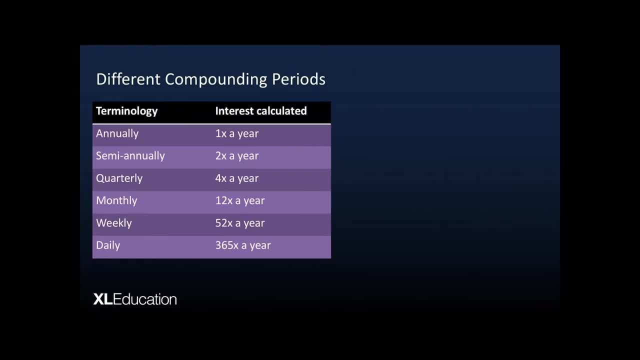 annually, Right? It means Right. Well, that till and 찍er log pi and'. So the answer here is a compound interest rate. Elar veya x Dad rad die lives hězaynol' means that interest is calculated once a year. Semi-annually would mean twice a year, quarterly. 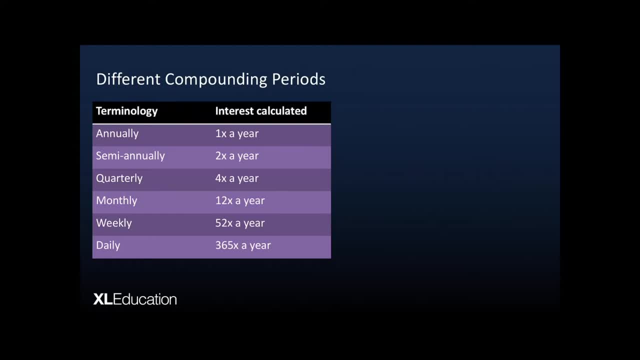 four times a year, monthly, 12 times a year, weekly, 52 times a year and daily 365 times a year. So we've got to be familiar with those terminologies there. So let's then move on and look through an example, And first, before we do that, we note that different compounding periods have absolutely 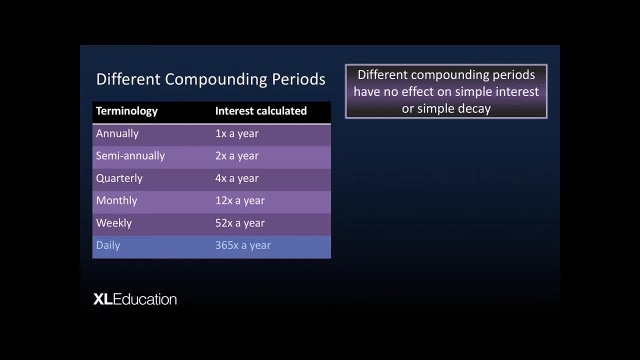 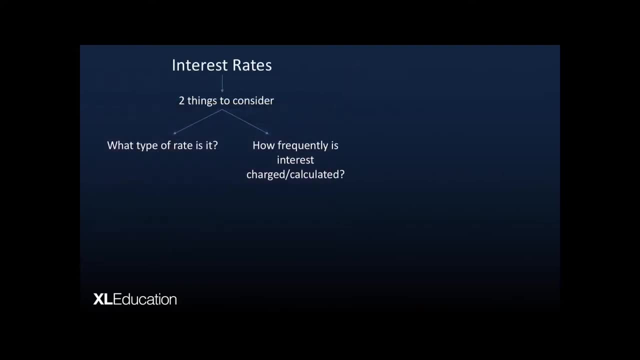 no effect on simple interest or simple decay. So it's only when we're dealing with compound interest or compound decay that compounding periods are actually going to have an effect, right? So if the type of rate is different to the frequency with which it is compounded, 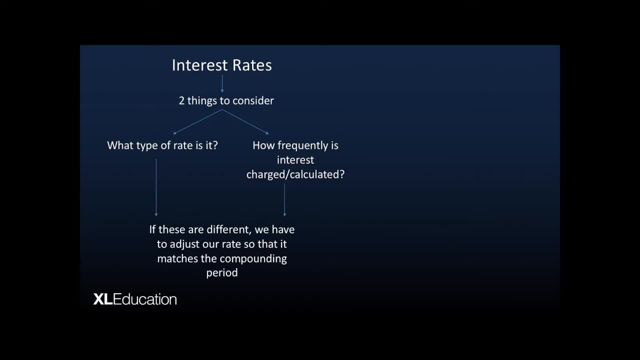 we have to adjust the rate so that it matches the compounding period. What do I mean by that? So if you've got an annual interest rate but you are compounding it monthly, you've got to adjust the rate so that it matches the compounding period. What do I mean by that? So if you've got 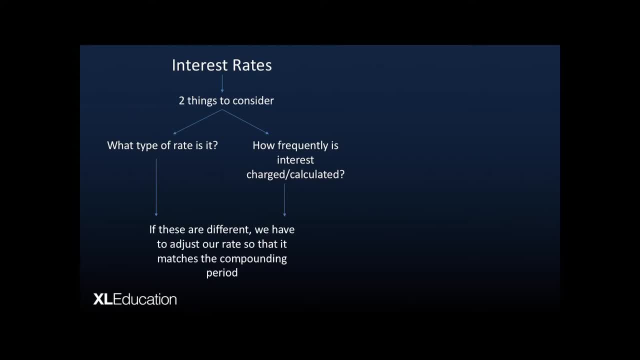 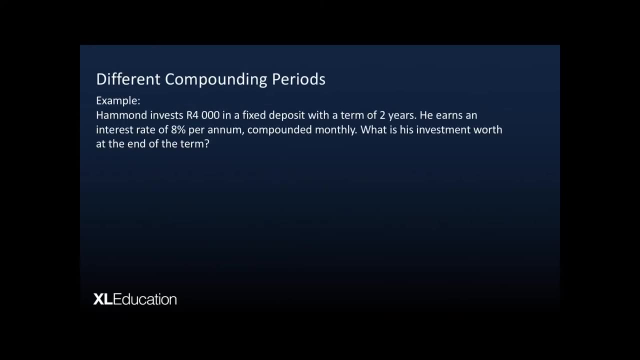 adjust that annual interest rate to turn it into a monthly interest rate, so that the interest rate matches the compounding period. So let's do an example. Hammond invests four thousand grand in a fixed deposit with a term of two years. He earns an interest rate of eight percent per annum. 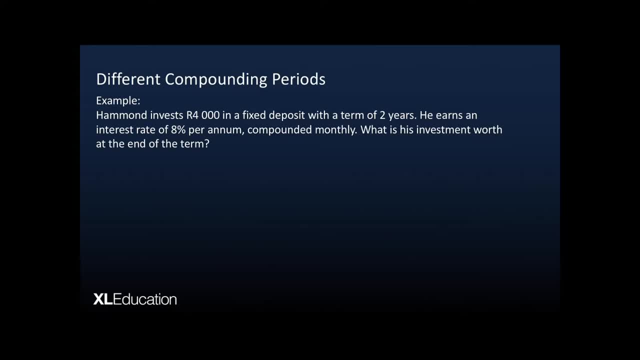 compounded monthly, What is his investment worth at the end of the term? Right? so we're going to represent this on a timeline and we know that we're dealing with two years, right? So we've got year one and we've got year two there, right, We're told that the interest rate is eight percent. 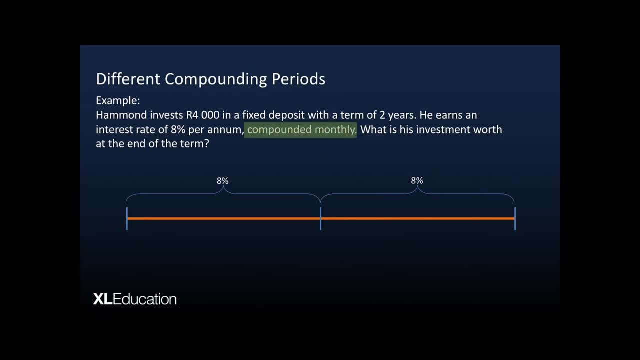 per annum. so we want to earn eight percent each year. but then it says that it's compounded monthly, which means that interest is going to be calculated each month. So we've got to take our year and we've got to break it up into the 12 months, and in the first month we find that we can't charge a whole. 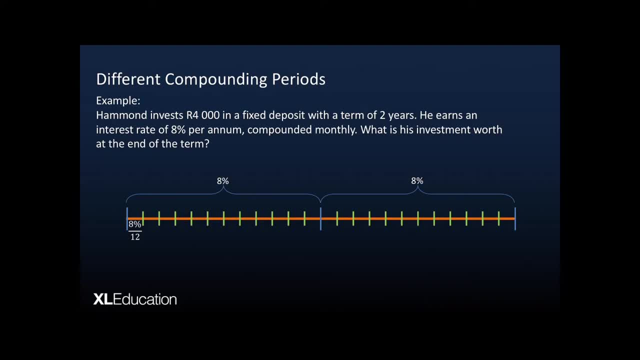 eight percent. we've got to charge eight percent divided by 12.. So we've taken 8% divided by 12, so we've taken 8% divided by 12. so we've taken 8% divided by 12, so we've taken. 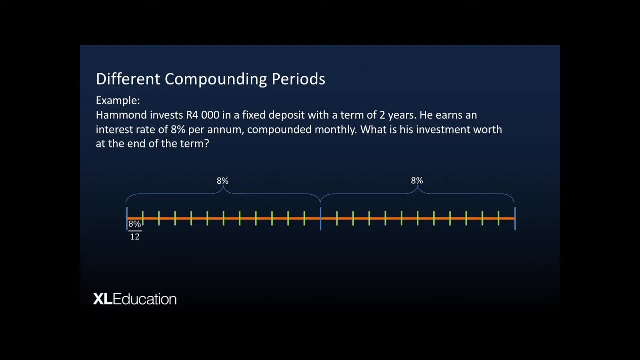 our annual rate and we've turned it into a monthly rate by dividing by 12, and then in the next month we also have to charge 8% divided by 12, and it continues like that, so that in each and every of the 24 months we are charging an interest rate of 8% over 12, because then our compounding period 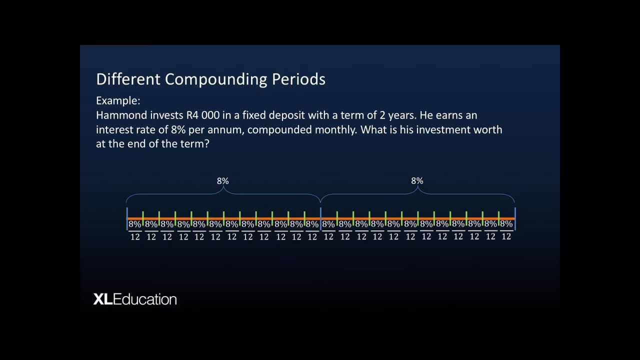 which is monthly, matches the interest rate, which is now a monthly interest rate because we've taken our annual one and divided it by 12.. So now each year, instead of just charging 8%, we are charging 8% over 12, 12 times right, so that our interest rate becomes 8% over 12 and our number of periods 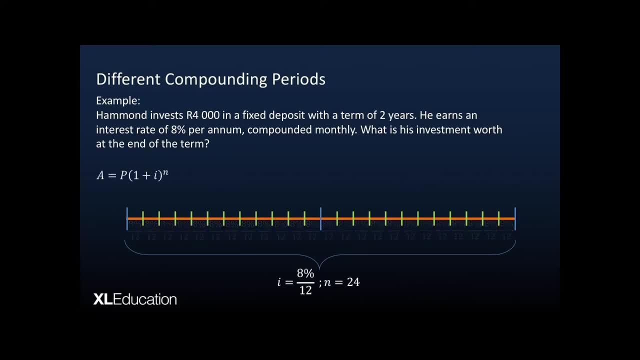 is going to be equal to 24, right? so then we plug that into our formula, right? our principal is the 4000, right? our interest rate becomes 8% over 12 and two years becomes 2. times 12, so that it's 24 months, right? so everything has been adjusted to reflect the 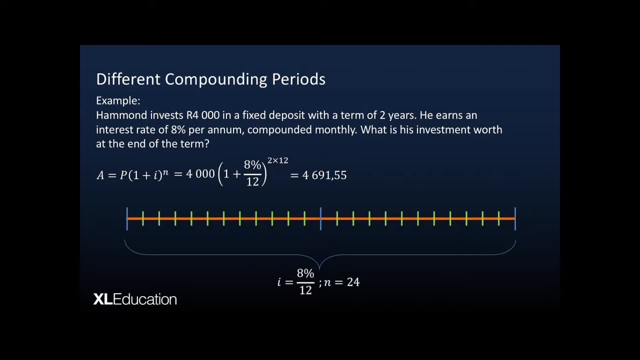 fact that we're compounding monthly, so our periods is counted in months and our interest rate is now a monthly interest rate and we find that Hammond gets 4691 rand and 55 cents at the end of that period. This leads us to an adjustment of our formula, so we've seen that a equals p, 1 plus i. 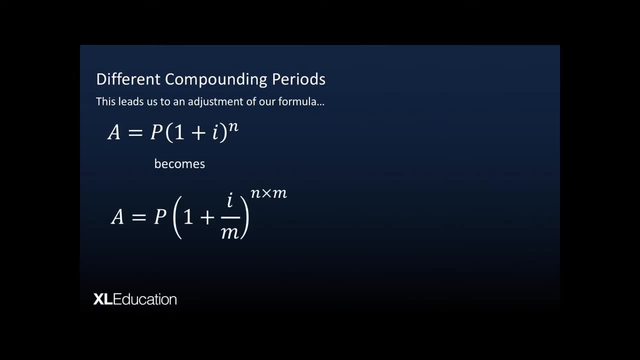 to the power of n, and that's what you're going to get. So we're going to get a 4.. you get on your formula sheet, but for you in your own mind, you can turn it into a equals p, 1 plus i, over m to the power of n times m. what on earth does that mean, right? so here m is going to be. 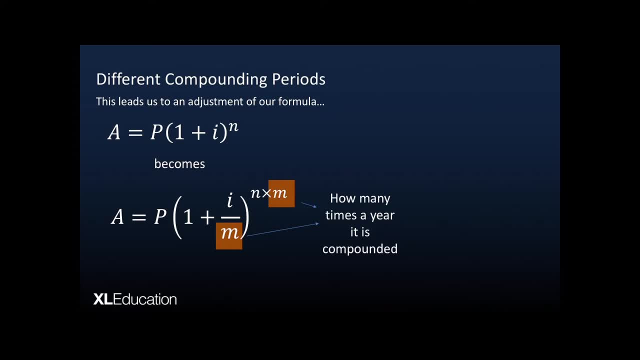 how many times a year it is compounded right, so that i there will usually be an annual interest rate right and that m will be how many times a year it is compounded. so if it is compounded monthly, then m is going to be 12.. if it's yearly, then m is 1. if it's weekly, then m is going to be 52 and that n there still remains. 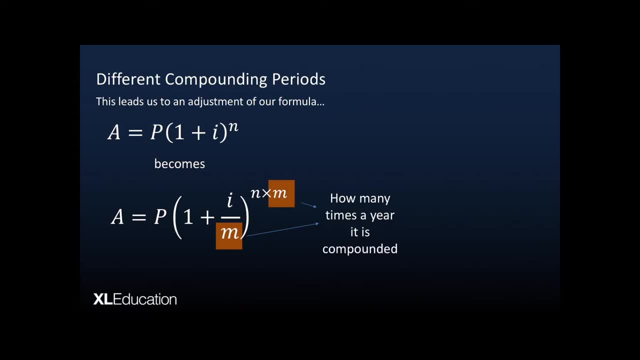 the number of years, but then n times m will give you the actual number of times interest is going to be calculated. so n times m is still the total of number of times interest is calculated. so let's look at an example. Joan invests 10,000 rand at an annual interest rate of nine percent compounded. 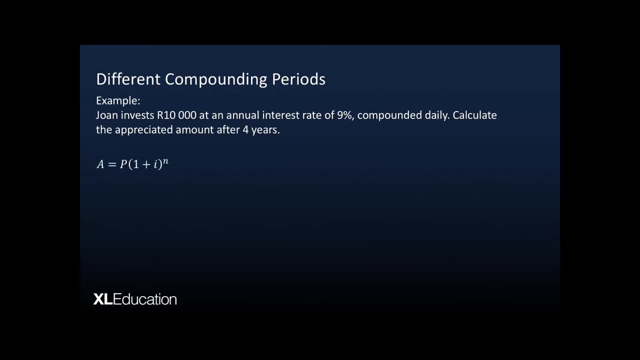 daily. So we've calculated the appreciated amount of the four years. so now we've got our formula there. but we know in our heads that even though the formula sheet says equals p 1 plus i to the power of n, we're going to adjust our interest rate so that it is a daily interest rate. so we take our 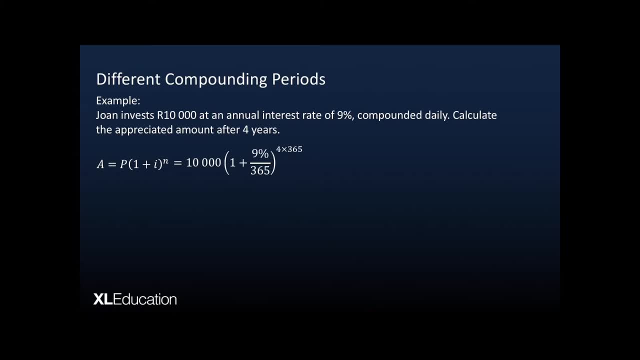 nine percent and divide it by 365, because it's daily. and we've got to take our four years and multiply by 365 so that the exponent becomes the total number of times that we calculate interest over those four years. Right? so there, just to highlight what we're talking about, because we're compounding daily. 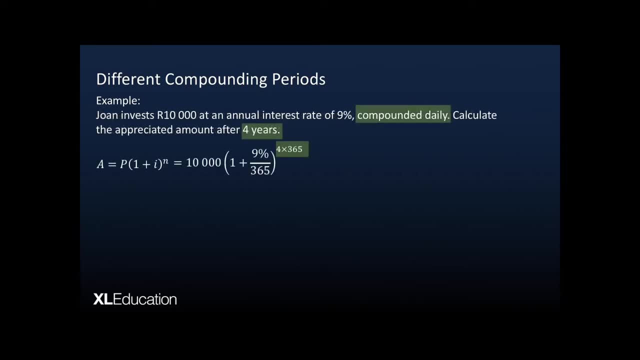 we've got to multiply by 365, and then that would give us the actual solution there right. another example: invest 10,000 rand at an annual interest rate of six percent, compounded quarterly, calculated the appreciated amount after three years. so here now we're compounding quarterly. so we've got to. 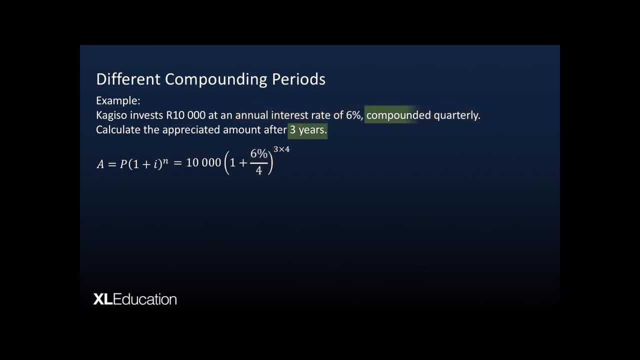 divide by four and we've got to take our number of times interest rate and we've got to divide by the number of years and multiply by four, because we're compounding quarterly and that'll give us the new appreciated amount. so how do different compounding periods affect the accumulated 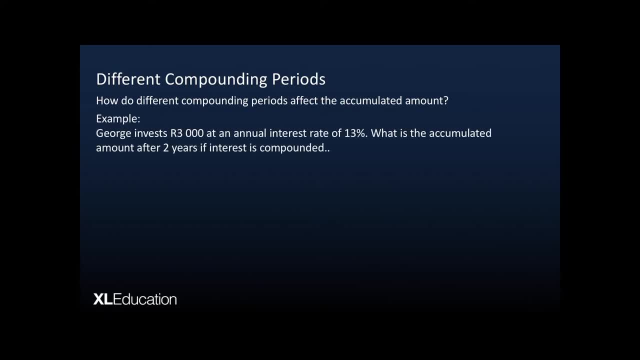 amount. let's see: George invests 3,000 rand at an annual interest rate of 13 percent. what is the accumulated amount after two years if interest is compounded annually, monthly or daily? so for annual, we're just going to use 13 percent over two years and we find we get 3,830. 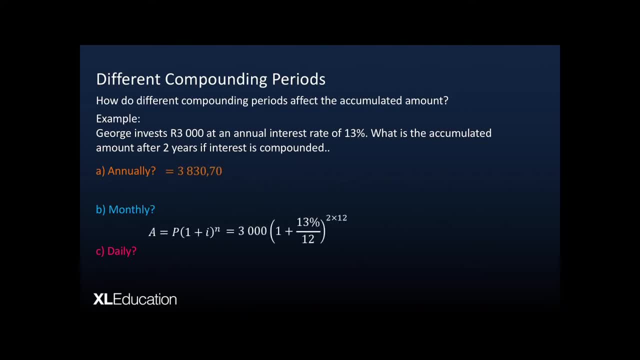 rand and 70 cents for monthly right. we now have to divide the interest rate by 12, but multiply the years by 12 as well, and we find that we get 3,885 rand and 35 cents as our accumulated amount. and for daily right we now have to divide the interest rate by 365, but our exponent is 2 times 365 and we 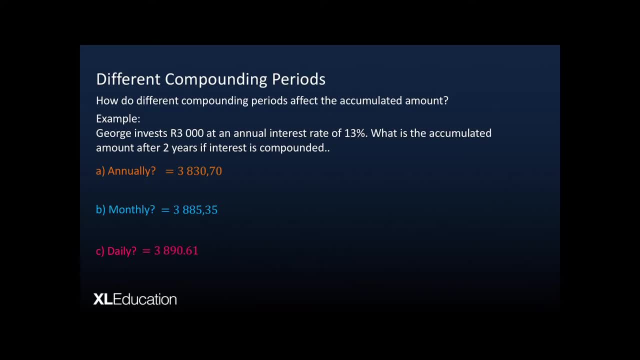 get three, eight, ninety comma six one. so what do we see there? it seems that the more frequently you compare the interest rate, the more frequently you compare the interest rate and the more frequently you compare the interest rate. but the thing that tends to shift is the ability to compound 방법ar. 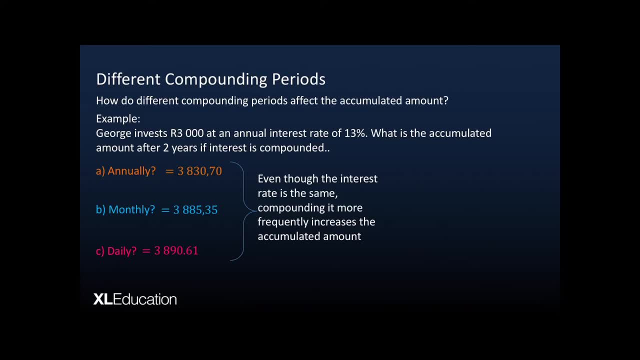 in one, three, three, three years. with compound algebra, the person who's compounding the interest rate, the higher the accumulated amount becomes. so compounding annually gives you less than when you compound monthly, gives you less than when you compound daily. so this is why the compounding 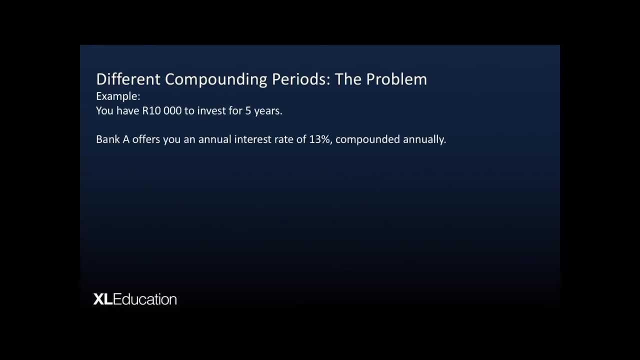 period is important. it actually affects the accumulated amount at the end of the day. but now we have a problem. let's say you have ten thousand rand to invest for five years. Bank Bank b offers you an annual interest rate of 12.5 percent compounded daily. now you know that. 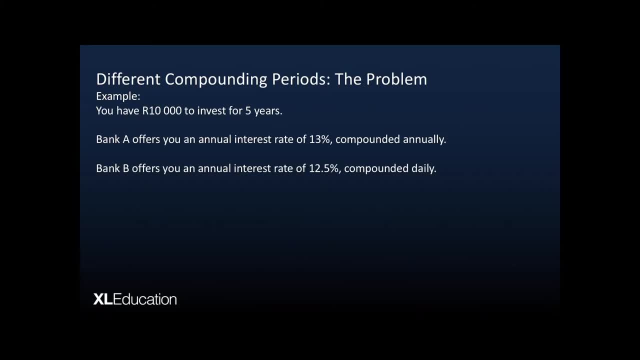 compounding daily gives a higher amount than compounding annually. but now the annual interest rate is higher than that compounded daily interest rate. so which one's going to give you a higher accumulated amount? well, without doing any sort of calculation, we just don't know, right. so we've got. 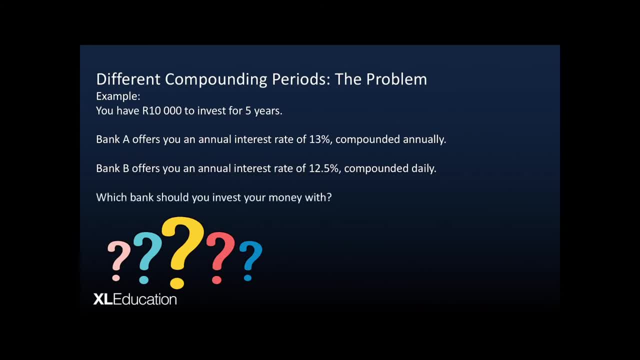 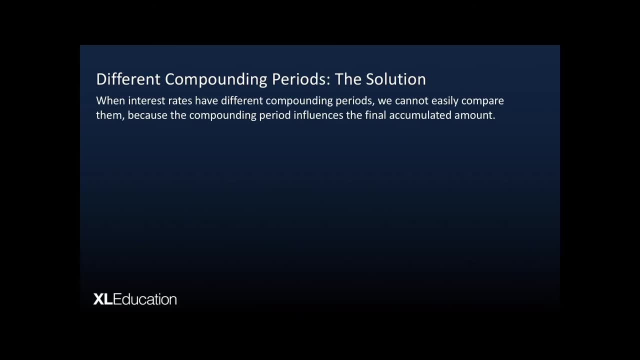 to find out which bank is going to be the best to invest our money with. so when interest rates have different compounding periods, we cannot easily compare them, because the compounding period influences the final accumulated amount. to make a comparison, we must find out what annual interest rate, compounded annually, will give us the same accumulated amount as the interest rate that 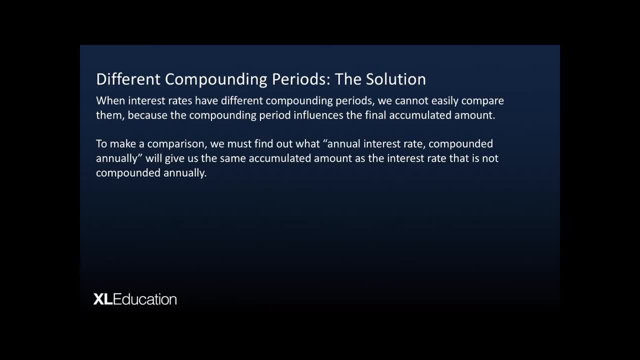 is not compounded annually. so we want to find a compound that annually calculated, once a year interest rate that gives us the same outcome or the same effect, the same accumulated amount as our interest rate that is not compounded annually is going to give us. so let's see: bank b offers us an interest rate of 12.5 percent compounded daily. 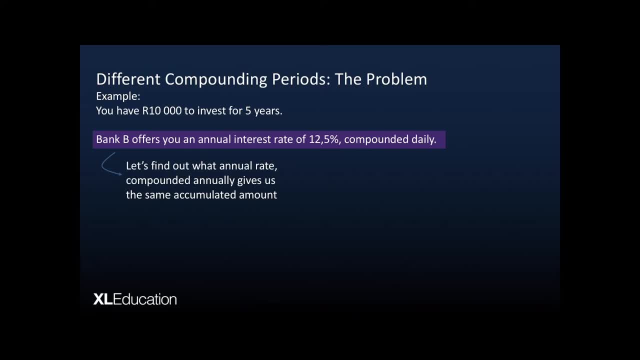 so let's find out what annual rate compounded annually gives us the same accumulated amount, right? so we know, in order to calculate the accumulated amount, we've got that formula there. but then if we just want to use i, an interest rate that is compounded annually, right, we've got to write the expression like that. but we know that we want both of them to. 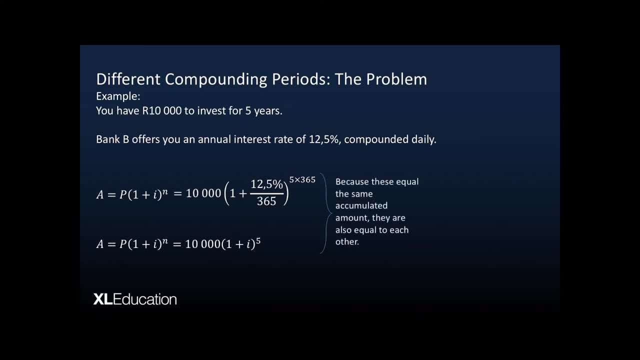 accumulate to the same amount. so we are just going to equate these two to each other, like we've done there. so now we've got a missing variable, i, and i is going to be the compounded annually, which gives us an interest rate compounded annually, which gives us the same outcome as this: 12.5 compounded daily. 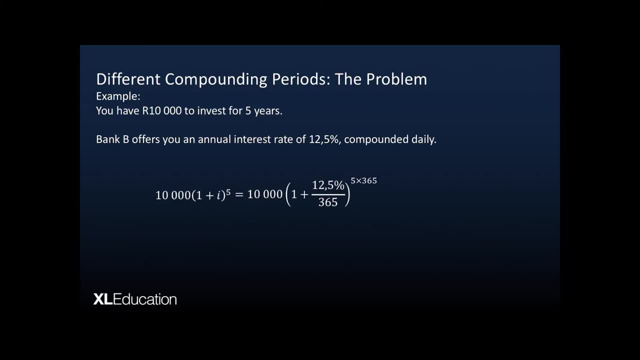 right and some terminology there that i. the compounded annually interest rate is going to be called an effective interest rate, because it gives us the same effect as that 12.5 divided by 365, which is not compounded annually, it's compounded daily, so that compounded daily interest rate 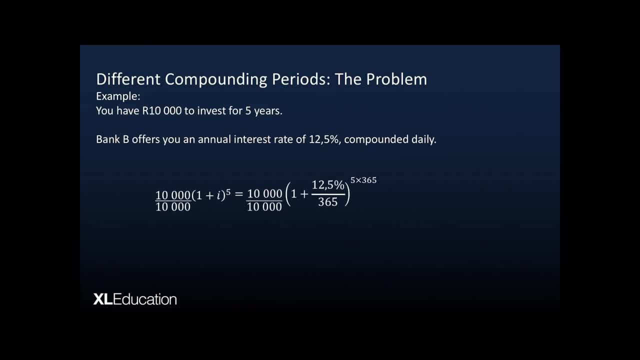 a nominal interest rate. So then we've got to divide both sides by 10,000.. Then we have to take this fifth root of both sides to get 1 plus i by itself, right, Then we've just got to simplify that exponent there, and we find this thing here, And what we found here is actually a formula that 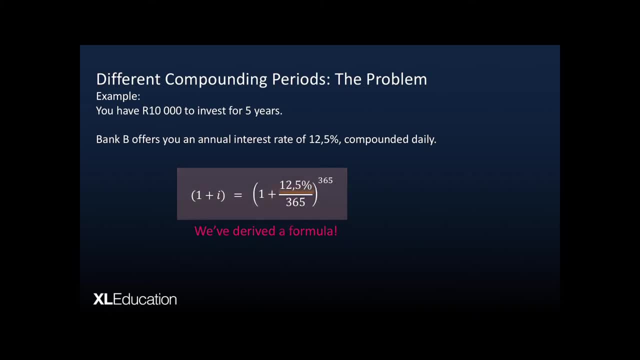 we can use to find the effective interest rate when we have the nominal interest rate, So that 12.5 percent is the quoted annual interest rate, That 365 is the compounding periods in a year And that i is the annual rate compounded once a year, that gives you the same effect as the quoted. 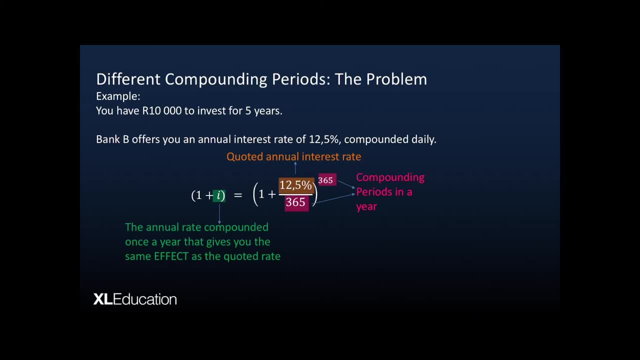 rate And we know that quoted rate is also called a nominal interest rate. So we are going to call this i the effective interest rate, So that i is the rate that gives us the same effect, the same outcome as the nominal interest rate. So we're going to call that i EFF in our formula. 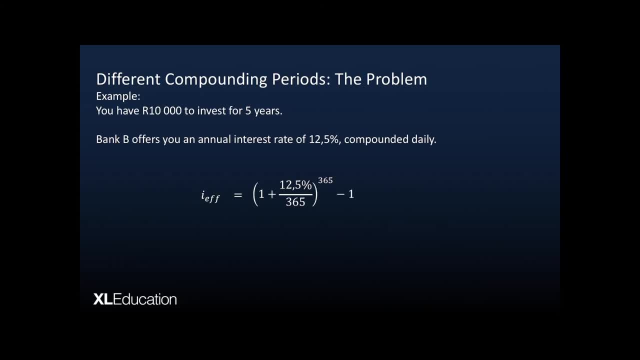 right. So now we just need to solve for i effective. We take the one across and we find that the effective interest rate there is 13.31 percent, right? So how do we use this to answer our question? Well, we now know that if we have a 12.5 percent interest rate compounded daily, 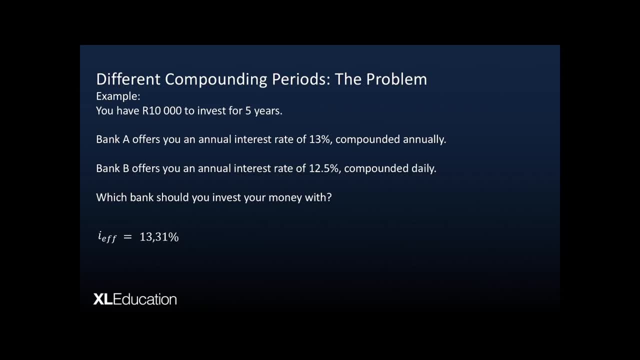 that's the same as having a 13.31 percent interest rate compounded annually, right? So the 13.31 percent compounded annually, which is what Bank B offers us, is better than the 13 percent offered by Bank A, So we should invest our money with Bank B. Now let's look at that. 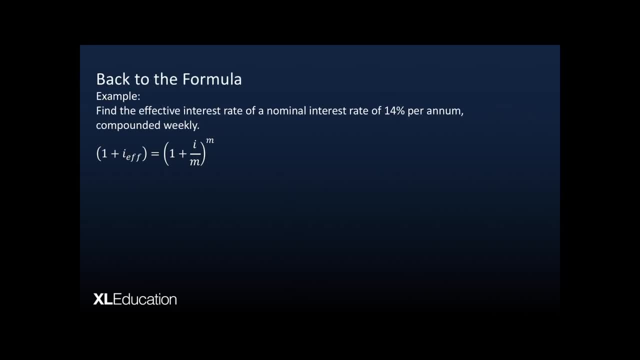 formula again right, We now know it's 1 plus i. EFF is equal to 1 plus i, over m, to the power of m, where m is going to be the number of times per year that that interest rate is compounded. So let's find the effective. 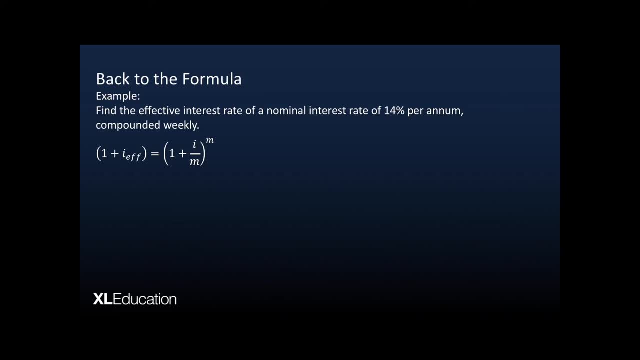 interest rate, of a nominal interest rate of 14 percent per annum compounded weekly. right So we've got 14 percent compounded weekly. so m is going to be 52, right So, our nominal interest rate compounded weekly. And then we take the one across so that we can find, i EFF, the effective.